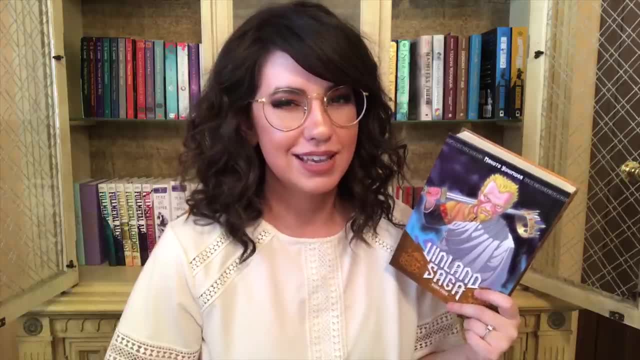 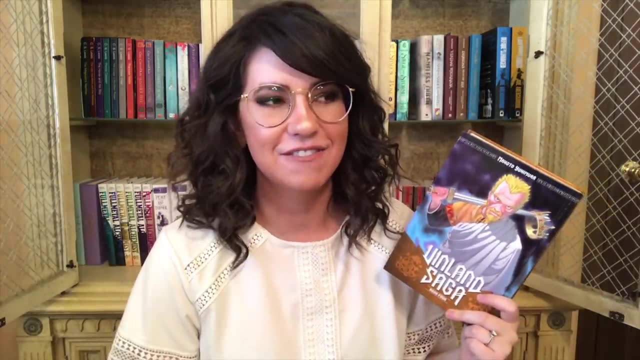 morally gray character is when you can make me care about them or at the very least I can kind of kind of get the- their motivations. I feel like with Askeladd as much as I'm like he's a terrible, absolute piece of. 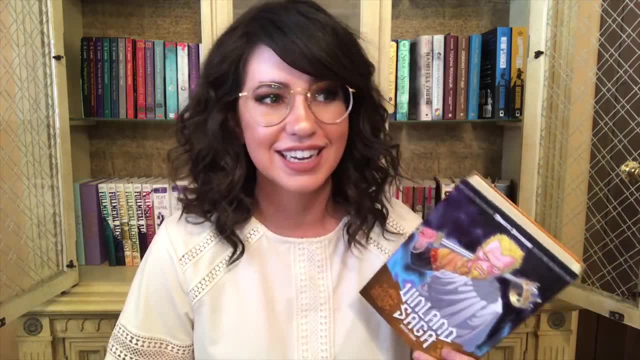 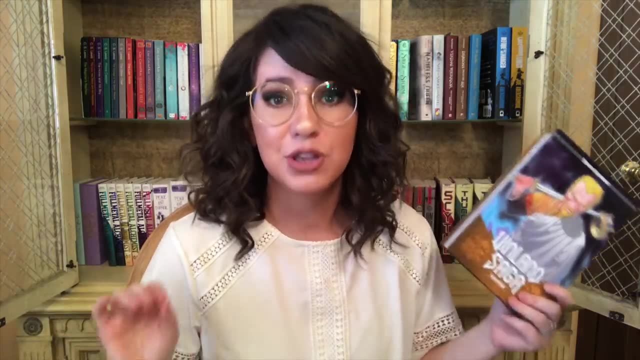 garbage I'm also like, but he's also really cool and kind of funny and I sort of see where he's coming from. sometimes Really good, morally gray characters are characters that if you end up liking them you realize suddenly you might be a terrible person, right? You're like I really 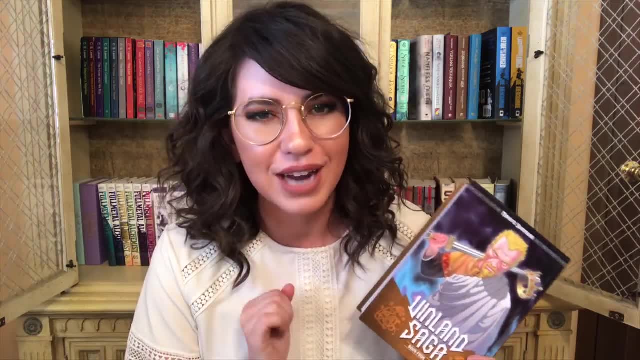 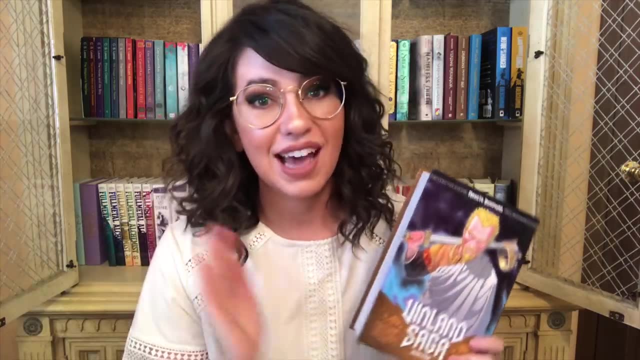 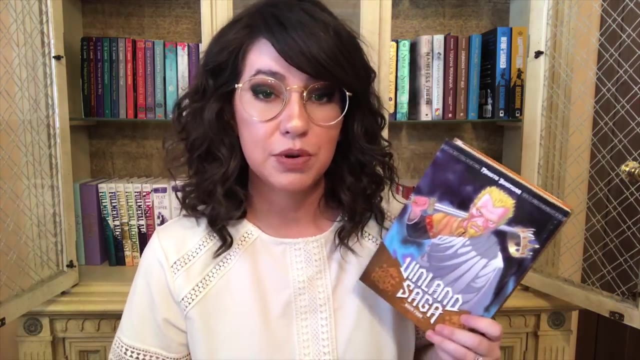 shouldn't like this guy. If I knew him in real life, I would hate Askeladd, but from a viewer slash reader standpoint, because there is an amazing anime, I would hate Askeladd adaptation of this. I just find him so fascinating. Vinland Saga is actually based around real people. 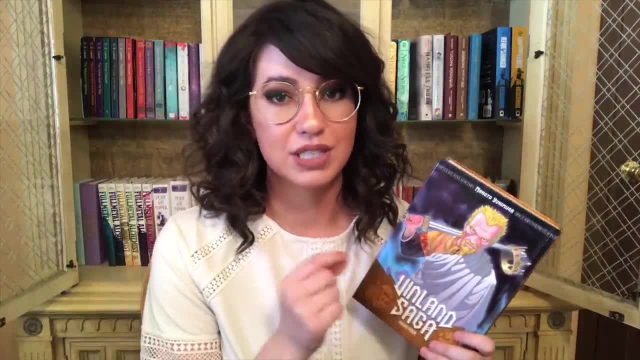 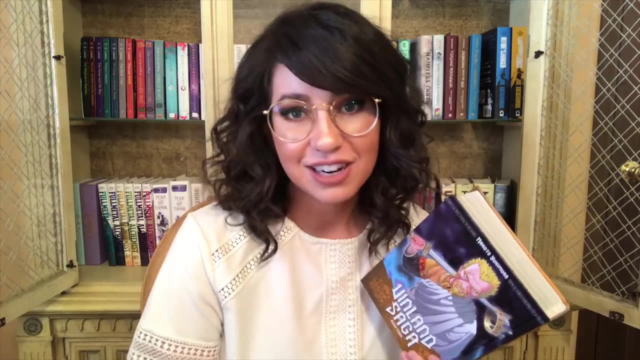 in history. It is a viking story. Askeladd was a real person. Of course, this is a fictional account, but it is based in history, which is kind of cool and adds extra layers to everything Next up, I feel. 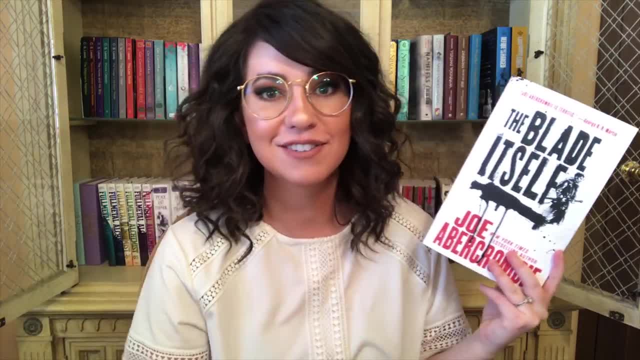 like. you can't talk about morally gray characters without talking about Glockta from the First Law trilogy by Joe Abercrombie. Truthfully, you could talk about basically any of the characters in this series. That's part of why I think it's so cool. I think it's so cool. I think it's so cool, I think. 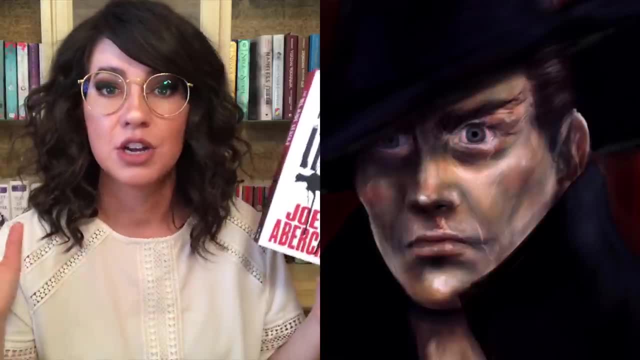 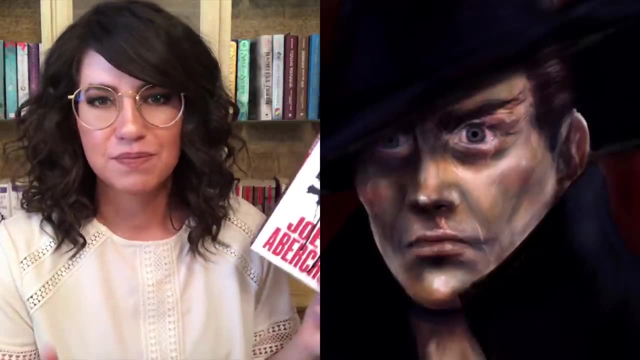 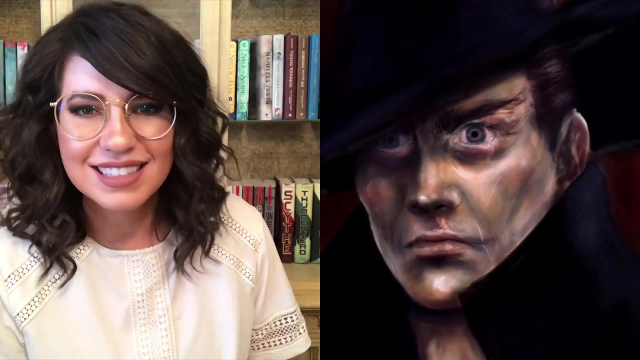 it has solidified itself as one of the grimdark greats. Glockta is a character who is somebody who interrogates people for the law to try and put criminals behind bars, if you will, or to get them to confess certain things. But what makes it so terrible is those interrogations often involve 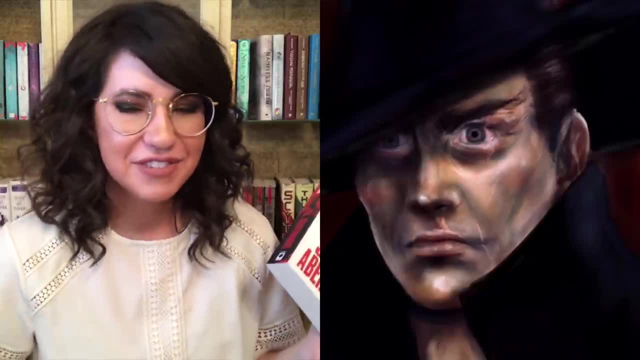 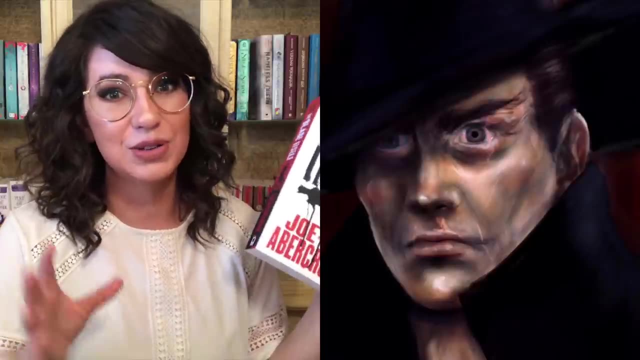 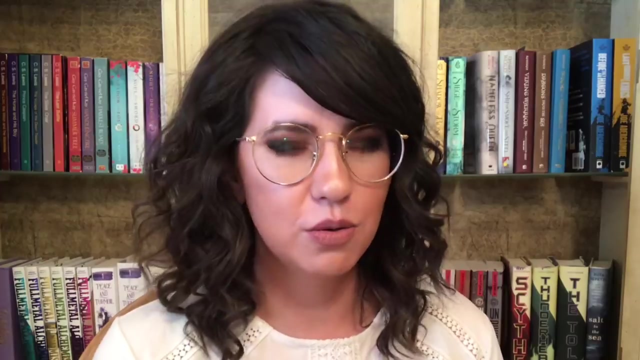 torture And also he often knows the people he's doing this to are innocent. Overall, for what he does, I didn't think it was over the top. And he's also such an extremely entertaining, fascinating character that you, kind of love slash, want to marry. I just want. I just want to be his. 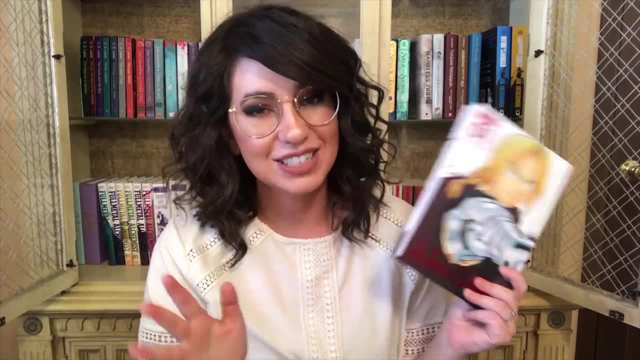 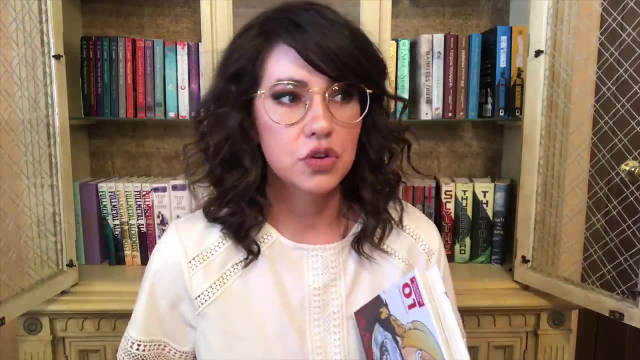 partner in crime. You know what I mean. The next one would be- I don't have the cover that has Scar on it, but Scar from Fullmetal Alchemist. This is a story that follows the two brothers who lost parts of their body, slash their entire body for one of them because of alchemy, Something. 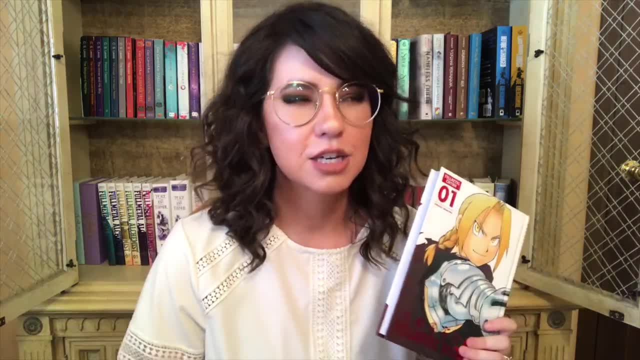 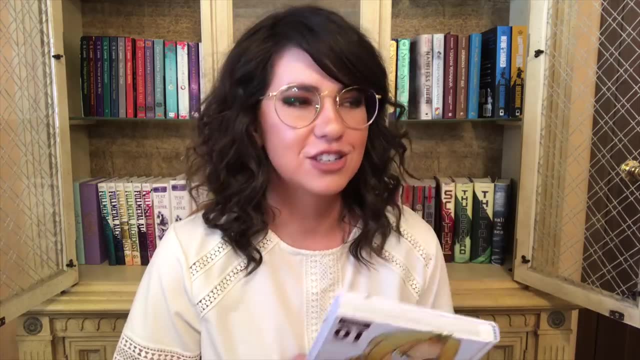 they're trying to restore their bodies, And so there are good guys. They're basically ultimate hero. I have to root for you because you're just so precious and wholesome. I love you so much. That's what the main characters are like, And then throughout the series you have varying degrees. 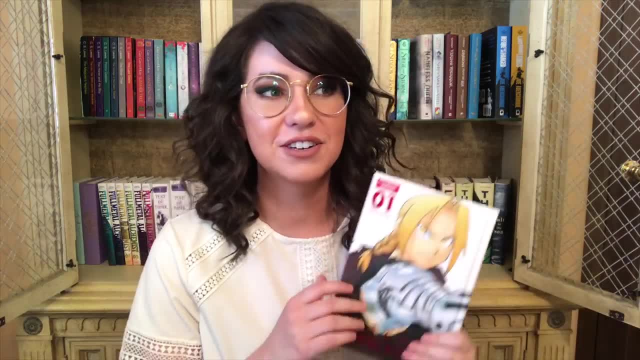 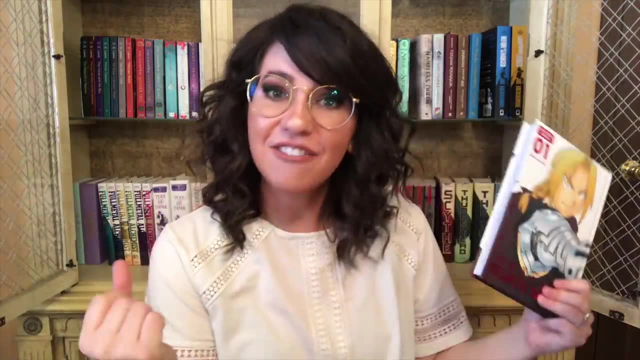 of evil, And Scar is one of those characters where, when you first are introduced to him, you're like this guy seems cool but also crazy, And then you start to just love him. Plus, he's super cool. Scar's the man. 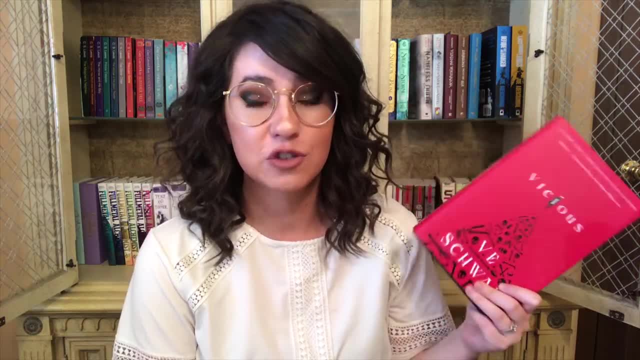 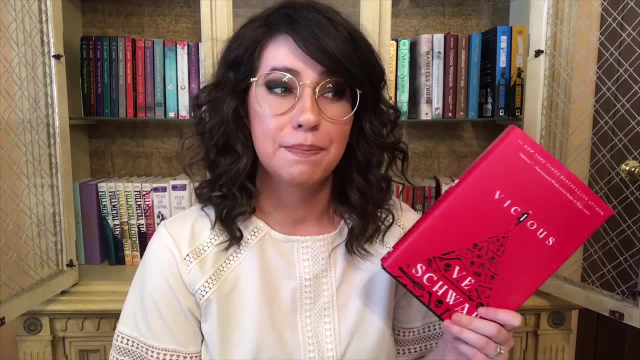 All right. So this is a story that follows probably pretty much any of the characters in Vicious and Vengeful by V Schwab. This is a story that follows people that are kind of like X-Men in a sense. They go through these experiences- I want to say near death, but they're not really near death. They 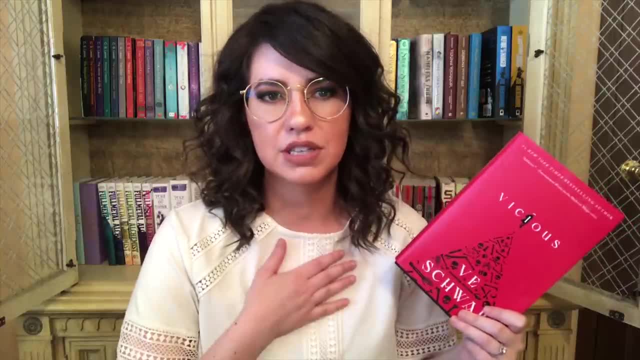 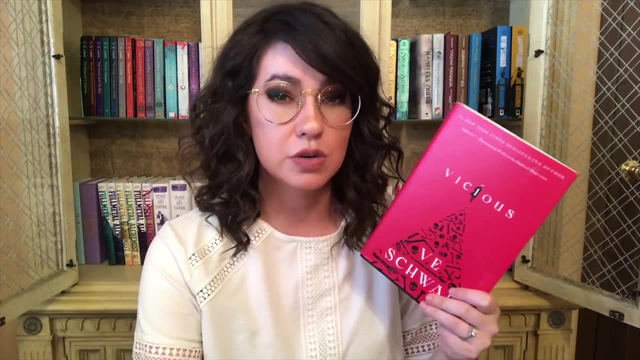 literally die, Then come back really quick, You know, almost like when somebody's heart stops, and then they get pumping again, that kind of thing, And then, as a result, these people suddenly have powers, but this isn't really known by society. All of these people discover these powers and 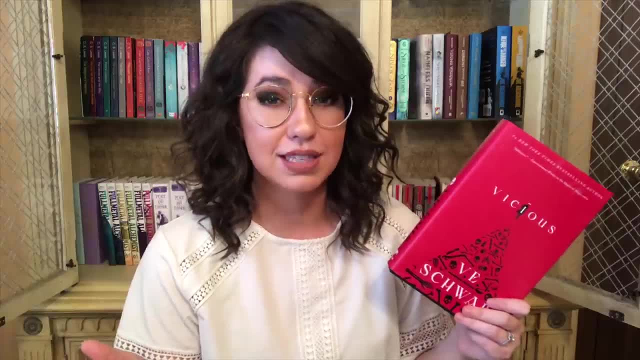 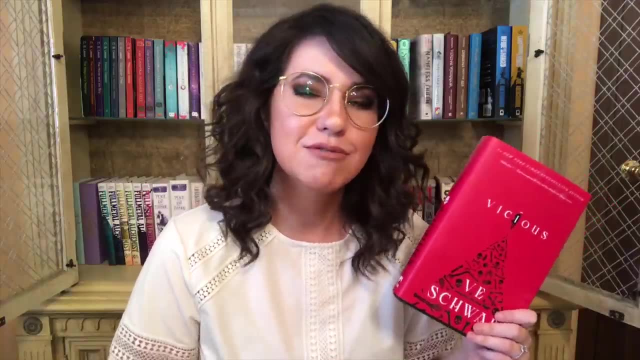 then now there's rumors that they exist, but most people think it's a myth. and we have two main characters who are like: I want to see if this is more than just a myth. I want to see if we can make this happen to us, And so they kind of 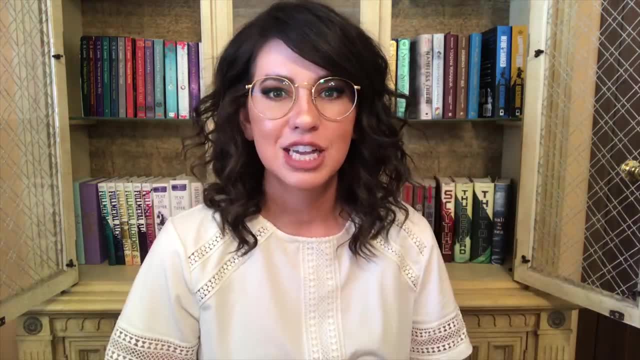 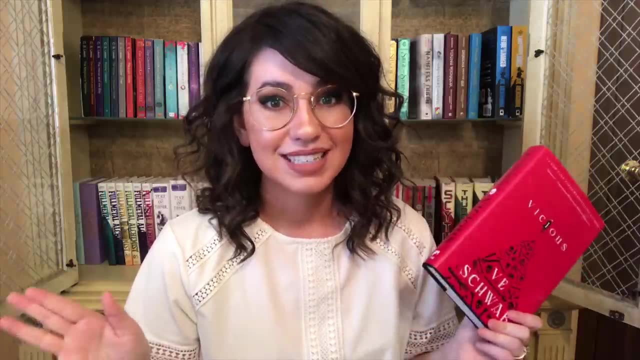 decide that they're going to attempt some science experiments to kind of kill themselves and then see if they end up getting powers as a result. From there stuff happens. You get a split timeline that I think is done masterfully, where you're not just getting past and present but you're 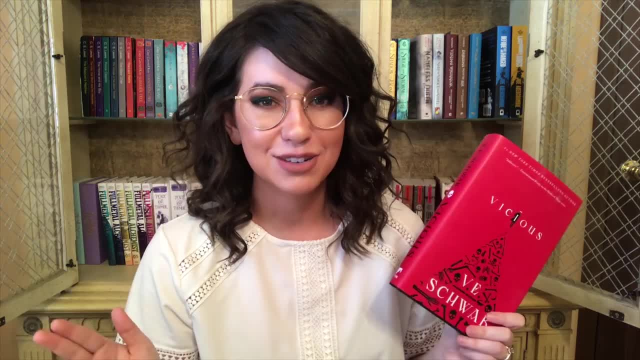 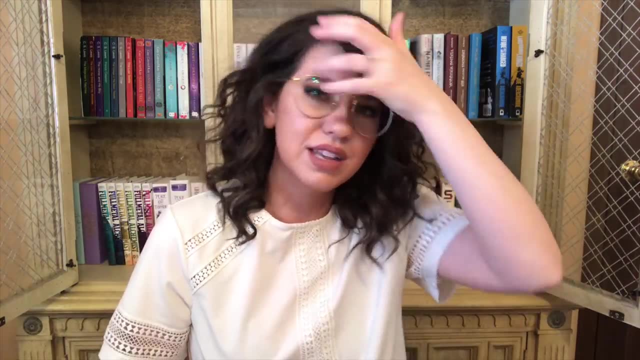 getting all sorts of different timelines throughout the story and everything starts to piece together and then the pacing towards the end is fantastic. I found myself in the first one being like: I like Victor, Victor's cool, Eli's crazy, Because in the first one you follow these. 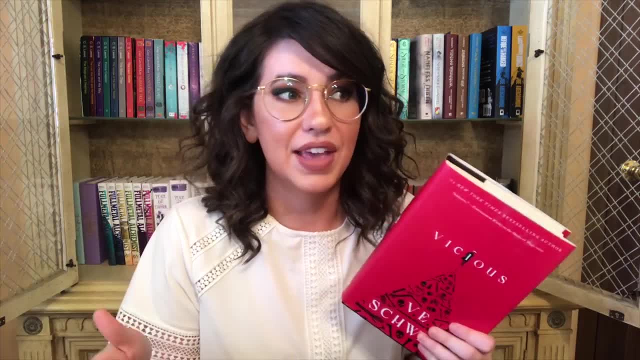 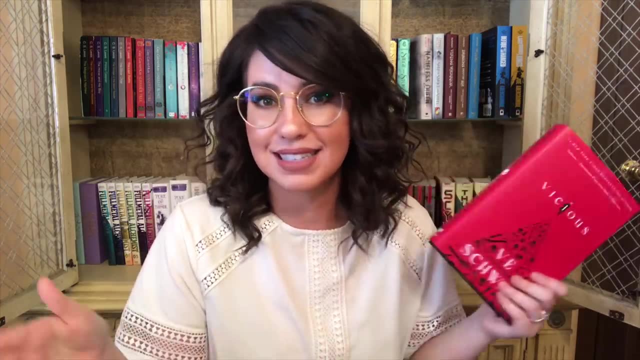 two characters that used to be best friends decide to try this experiment. and then you see later, now they hate each other and they want to kill each other And you're like, um, what happened? So you get the pieces put together as the story progresses. In the first one I was like: 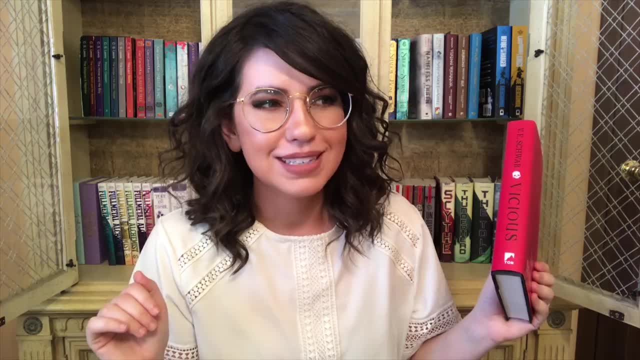 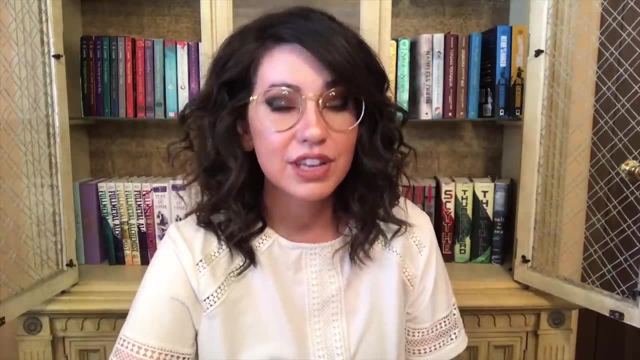 Victor's awesome. And then the second one. I mean Victor was always messed up, but in the second one I'm like: dude, how messed up do you have to be? Slash. I still, I'm still rooting for you Next up. we have a character that I feel like very few people. 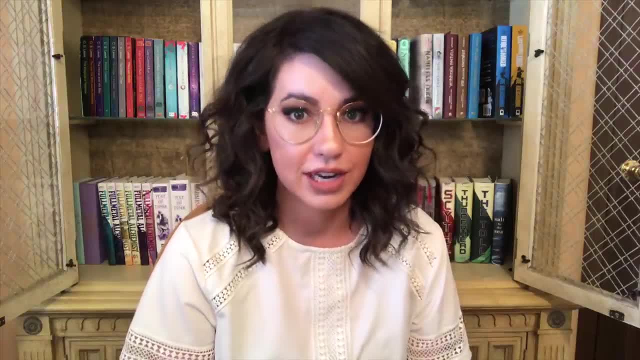 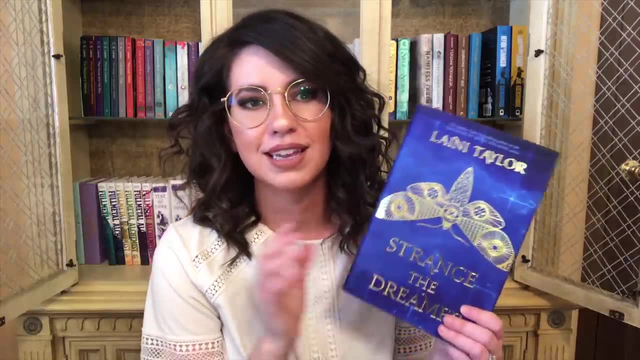 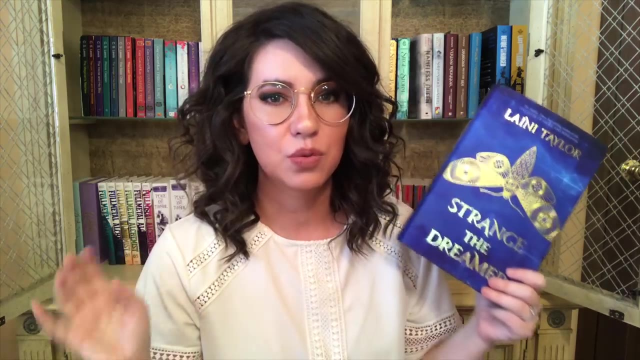 would actually think of this person when they think of morally gray characters, until they actually think of what this person did, And then they'd be like, oh yeah, that person's actually horrible. And that would be Errol Fane in the Strange the Dreamer duology by Laini Taylor. I can't really go into details as to what goes down. 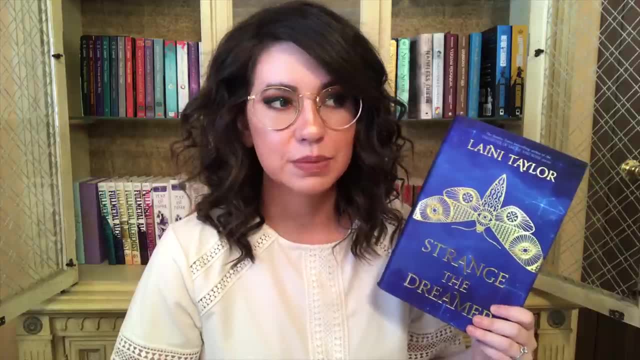 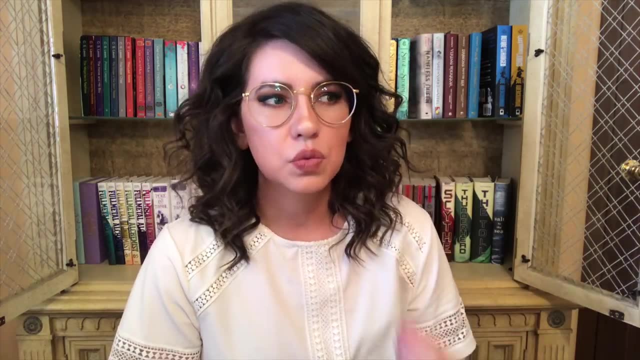 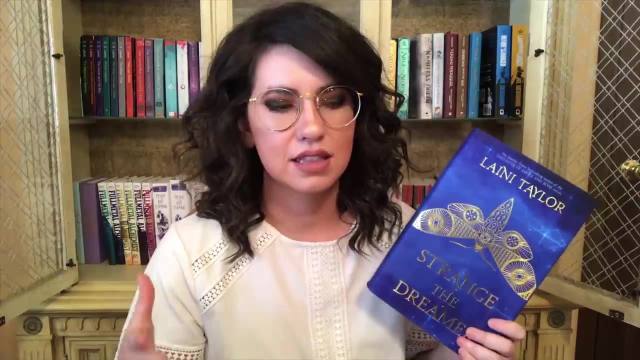 with Errol Fane, because I feel like the discovery of that is part of what makes this book what it is. But this is a story that it deals with so many extremely heavy themes, one of which- one of the main things- is: what? what do you expect a society do to do? What do you expect? 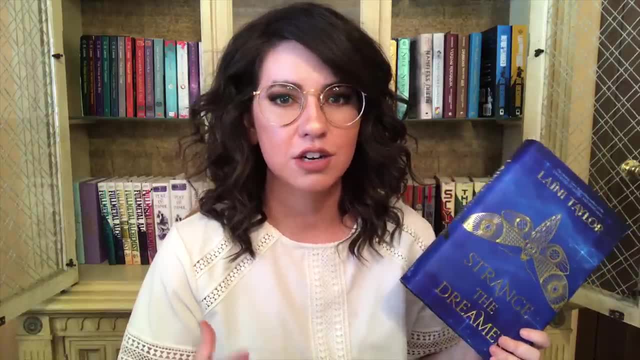 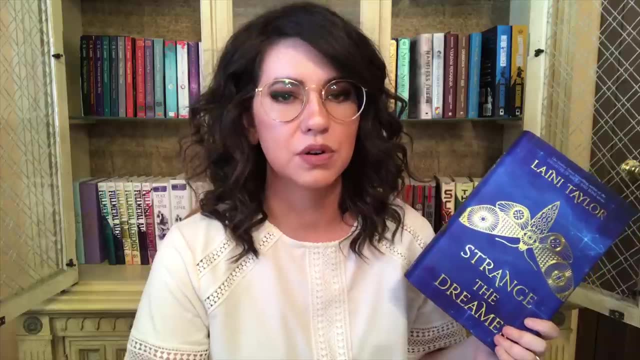 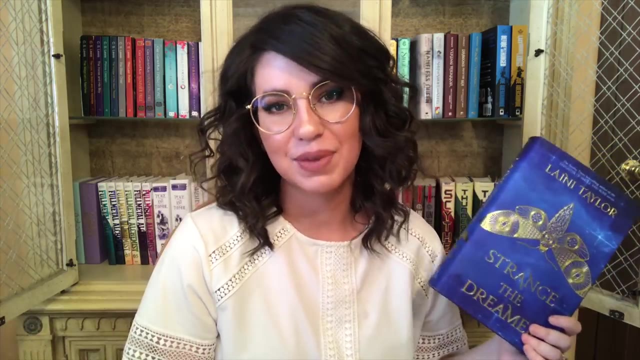 the people to do when they have been conquered and oppressed for years, And what is excusable for those people when they're attempting to get their freedom back? essentially, And how do you excuse some of the terrible atrocities they commit in the name of? finally, 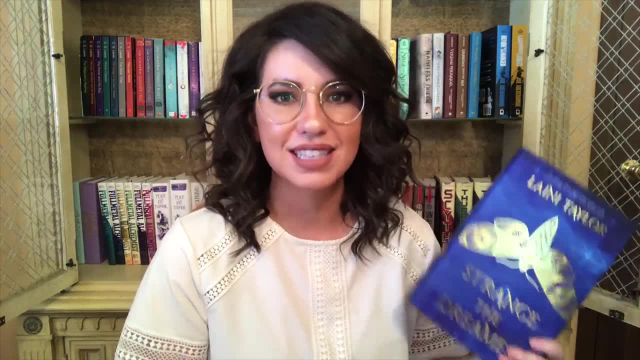 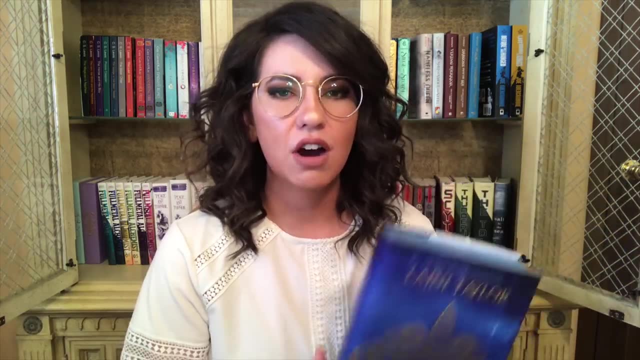 not being oppressed, right, That's what. that's what we see with this character, And I don't want to say what he does. I don't want to say what goes down, of course, but I just think that I constantly had to rationalize in my head: oh but, but this happened. And also the magic of the story, it like 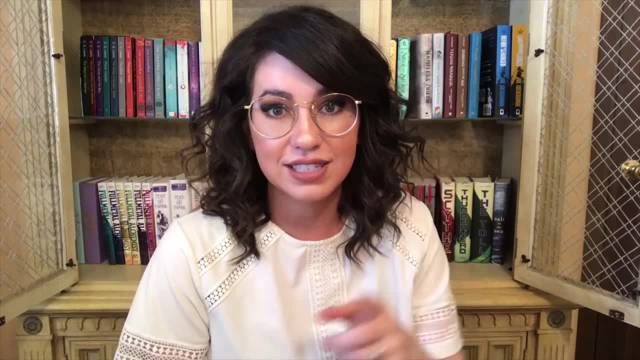 messed with his brain, And I think that's what I'm trying to do. And I think that's what I'm trying to do, Which could be true. you can also have theories as to was he influenced by magic, Was he not? Was? 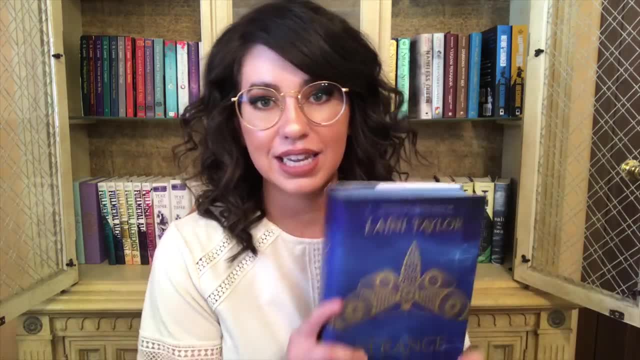 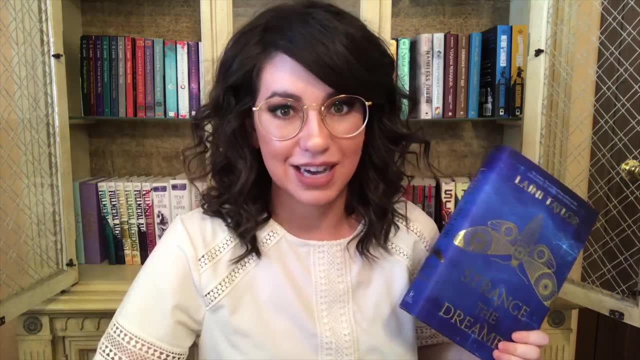 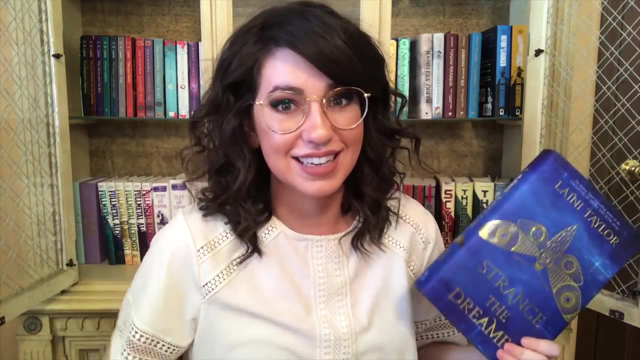 he just so done with all the evil, terrible things that were happening to him and his people. There's a lot of different ways to look at it, but I found myself constantly I needed to tell myself like oh no, this is how it was to justify the things he does, Because otherwise, like he's a horrible. 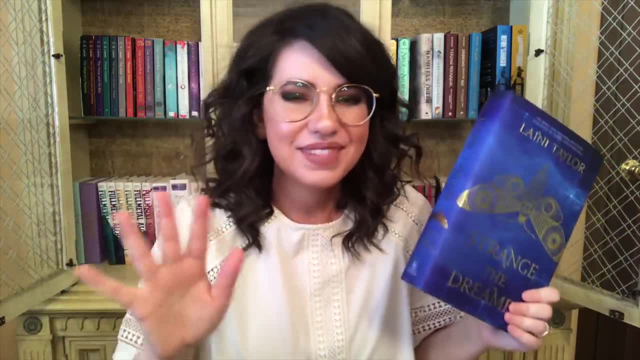 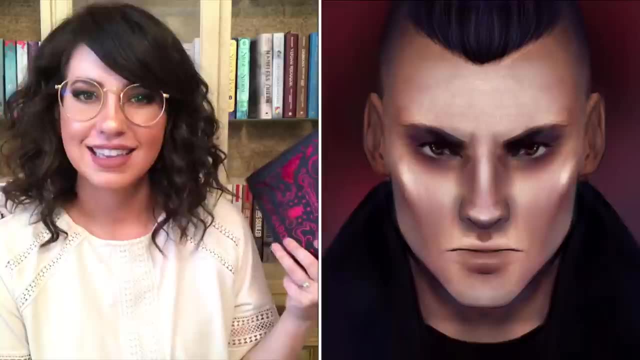 person. But then it's like: but is he? It's? if you read the story you'll understand. Next up we have Kaz from the Six of Crows duology by Leigh Bardugo. Kaz is like the edgelord of all edgelords, right, He's like. I'm edgy. I have like the shaved sides of my head. 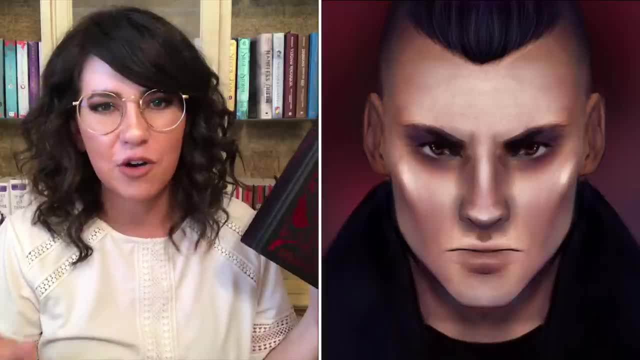 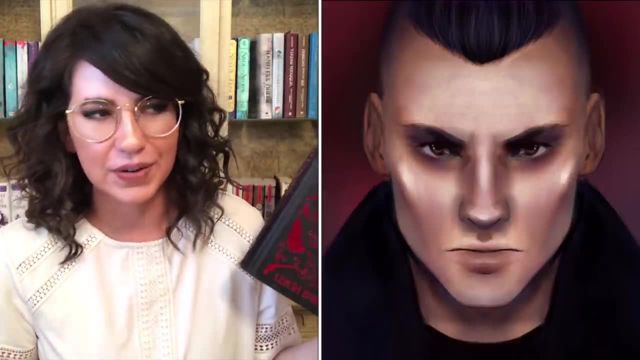 with the dark slick back black hair. He's just got that whole vibe. He dresses in dark clothes and he's got like his cane. He just has this whole look and this whole persona And you're like, oh, it's just a lie, right, Like he's actually a softie, Except for he's not. He's really not, He's. 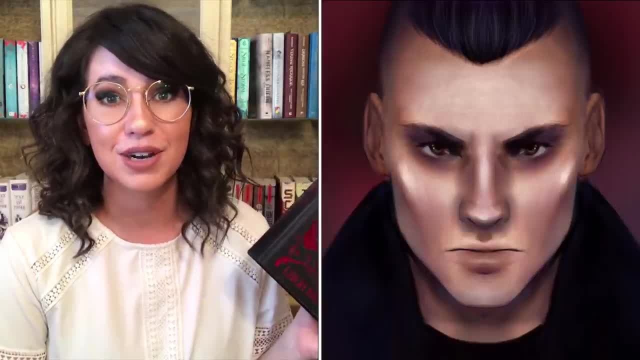 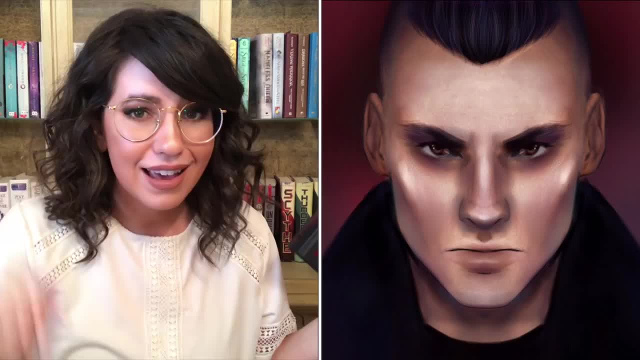 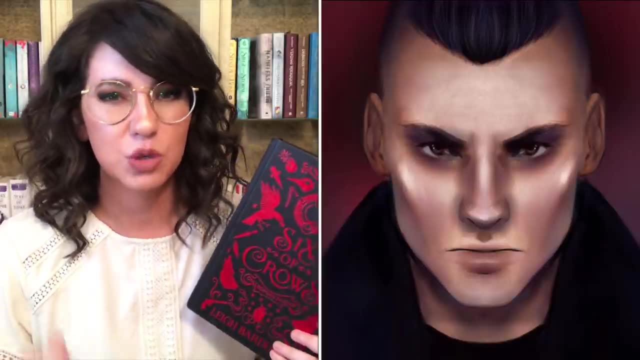 point, just like ripping somebody's eye out of their head, which I don't even like saying because I have an eye phobia. So that part I was like I can't read this part. He's willing to do what needs to be done to get what he wants. And what he wants sometimes isn't necessarily like I just 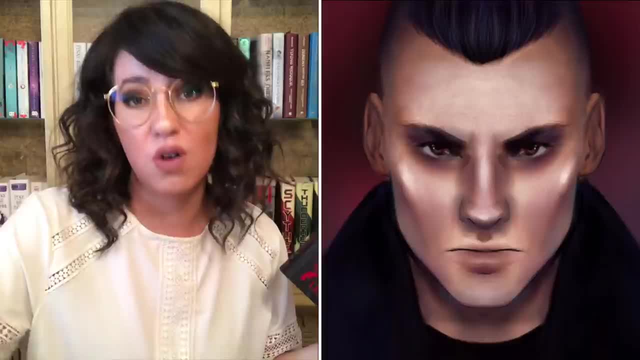 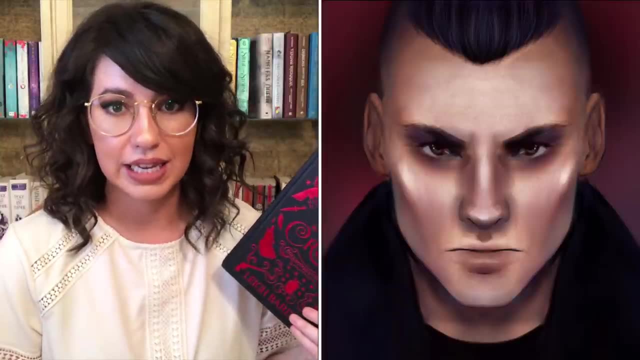 want good for everyone. He's like: no, I want what I want. Of course that makes him sound like he's a straight up villain. He's just a terrible person. But when you dig deep into why he is the way he is and some of his motivations and the things, 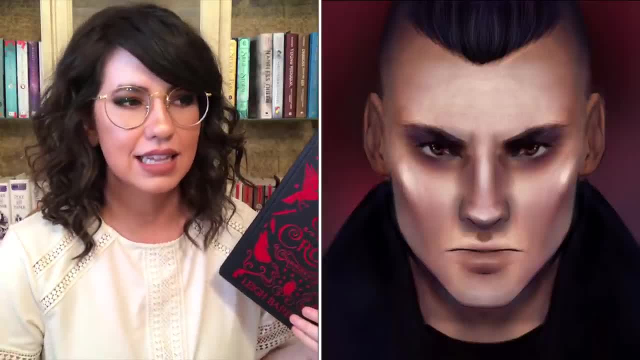 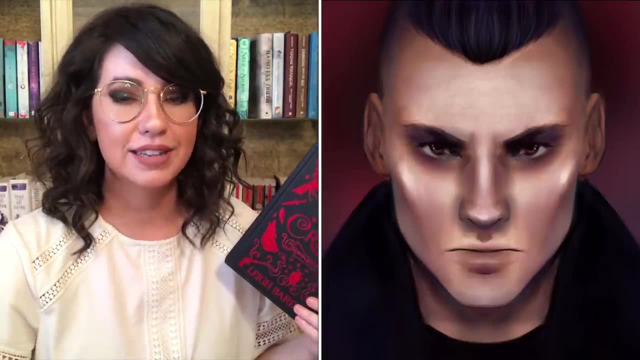 he's struggling through, you start to kind of see why he's like that, And then I think that you start to see glimpses of a person underneath this exterior. but that exterior is kind of buried itself so deep that it's basically a part of him. now This next one. I don't think these characters. 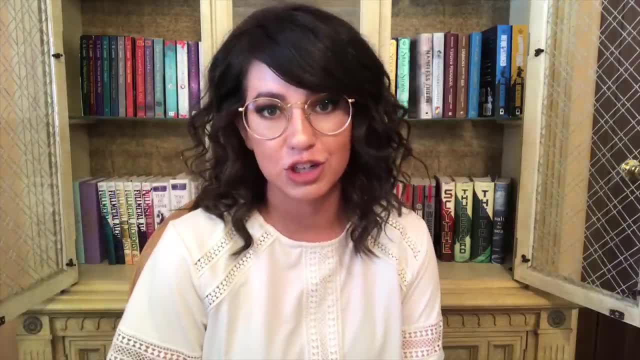 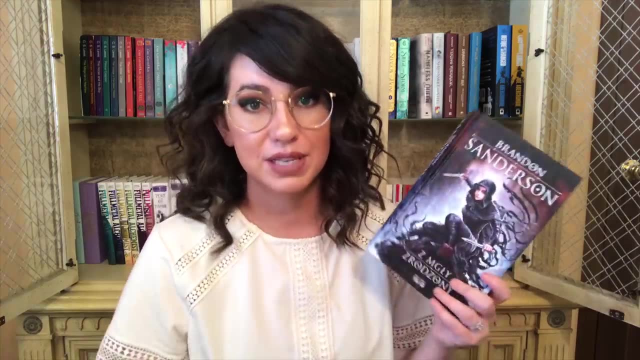 are really on the same level as a lot of the other people I have mentioned on this list, But I still feel like they're pretty morally gray. And that would be both Vin and Kelsier from the Mistborn series by Brandon Sanderson. Vin shows countless times throughout the story that 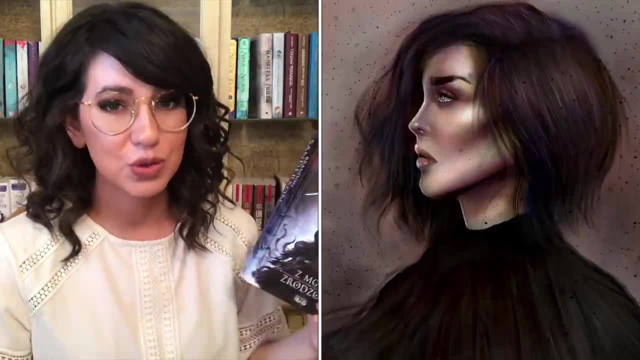 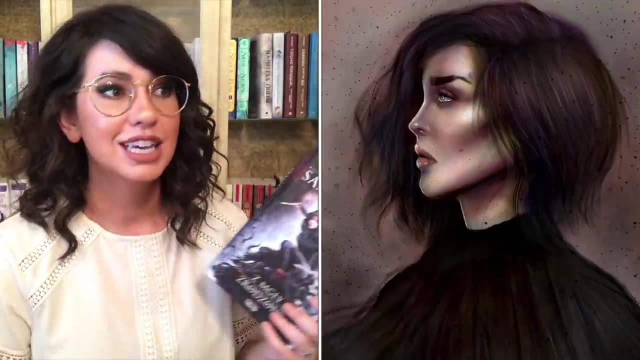 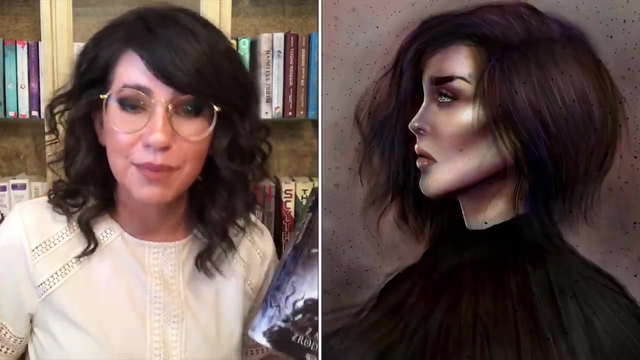 if she has to do something violent to protect those people that she cares about or for the greater good, she's gonna do it. So sometimes she ends up becoming a little extra paranoid and then is like: well, I think this person's a threat, so I'm gonna go kill them. 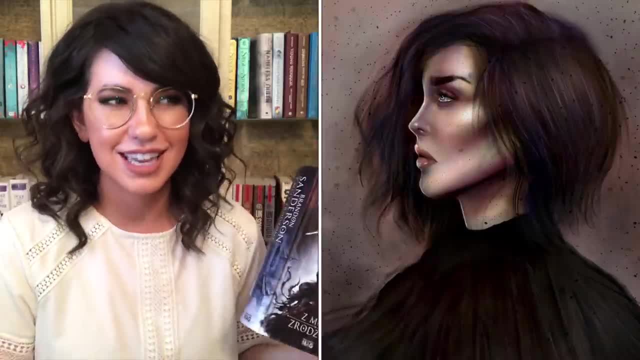 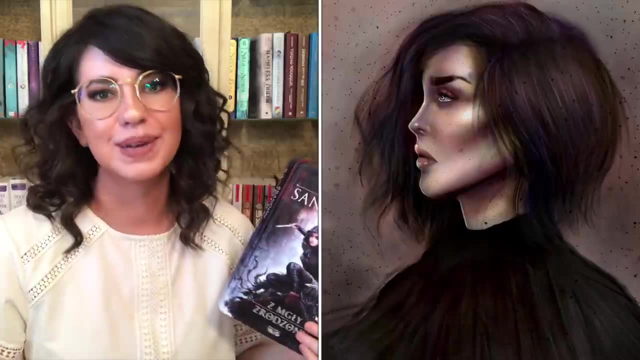 and she doesn't always figure everything out first. She's definitely got these violent tendencies, but she's still like. I think most of the time when we think about Vin, we think she's awesome, she kicks a lot of butt and she's cool. We just are like, ah, she's so cool, I want to be like Vin. 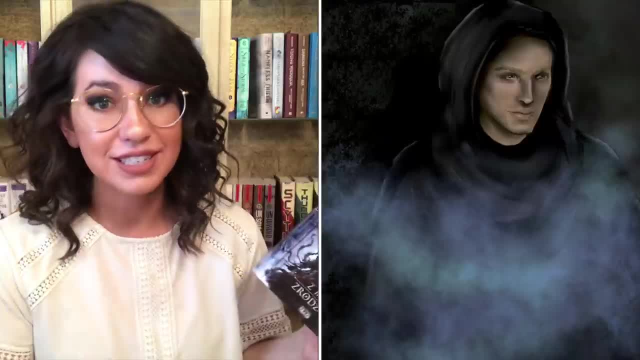 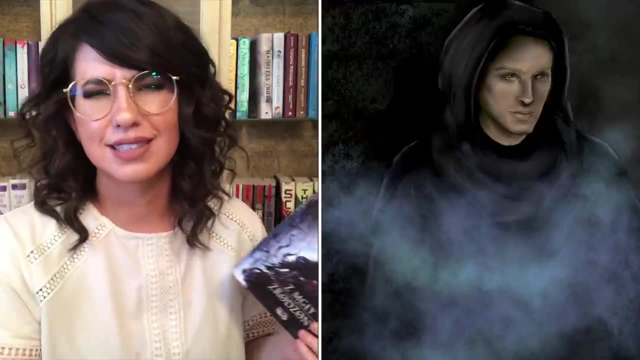 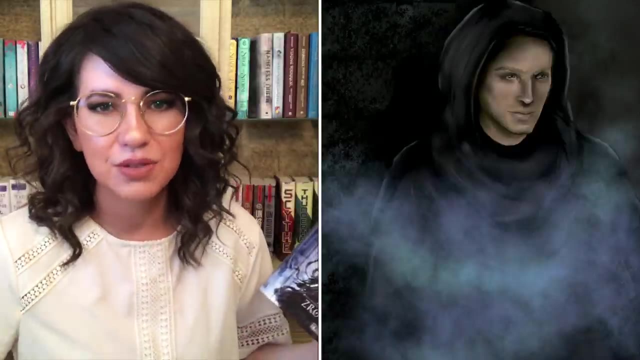 but Vin's got some issues On that same topic. Kelsier is this very charismatic, charming leader who wants to help the essentially like slave population of their world and you're like: what's behind that? That sounds great, Except it's like anybody who's on the other side in his eyes. 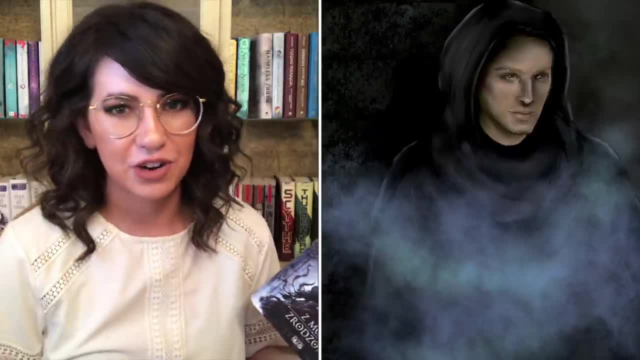 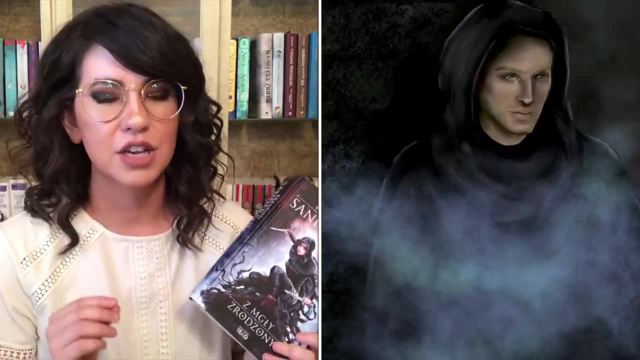 like all of them must be evil. He has this huge blanket over all of them and it definitely clouds his judgment at times, a lot of times, and it's a big part of his character, I think, to start to to see if perhaps that's the best way to go about it. I have one more character on this list and 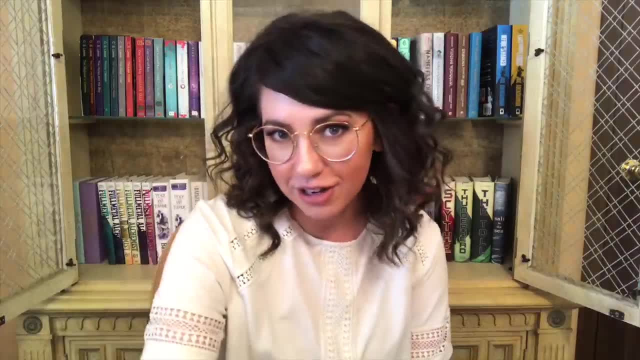 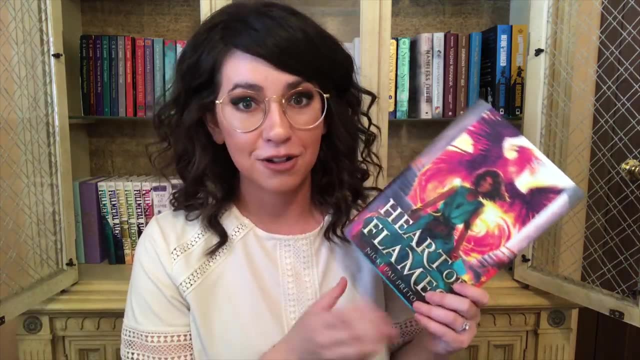 then I have an honorable mention that I feel like most people would have put on their lists, but I'll get into a little bit. The next one, the last official one, would be the character Val from the- this particular one, Heart of Flames, which is the sequel. I think it really shows in this one. 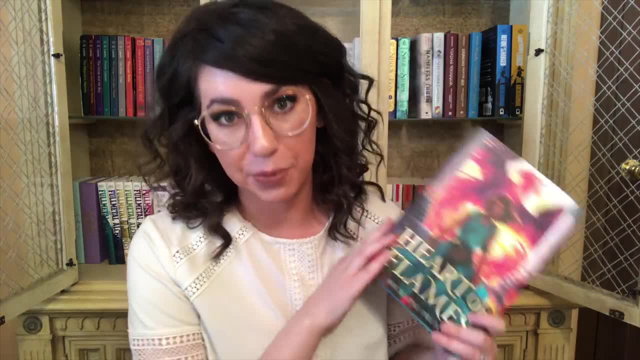 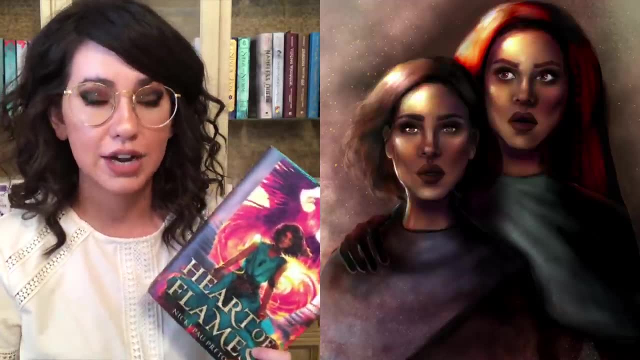 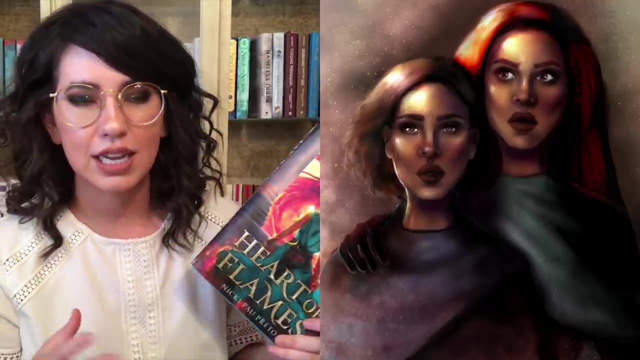 but also Crown of Feathers, is the first one. They're by Nikki Palpreto. This is a story that follows a girl who has dreams of having her own phoenix and becoming a phoenix rider. Phoenix riders were essentially exiled from their homeland, and people with any kind of animal magic are seen. 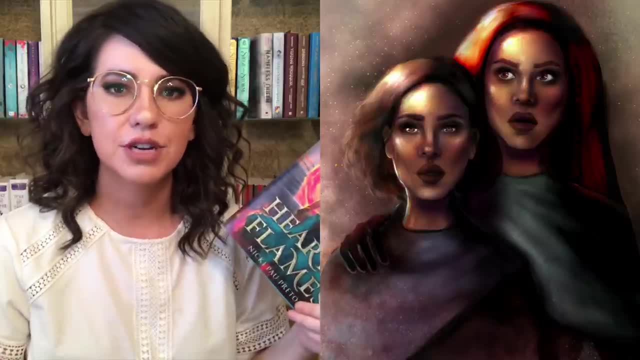 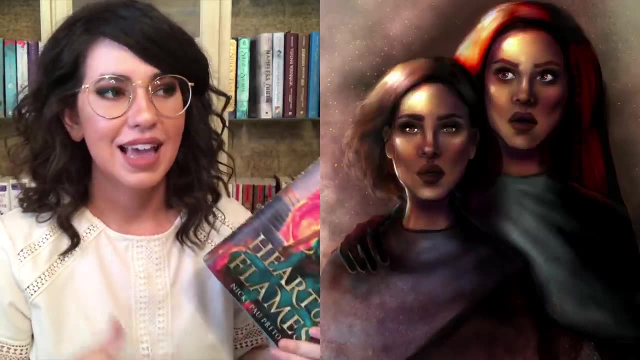 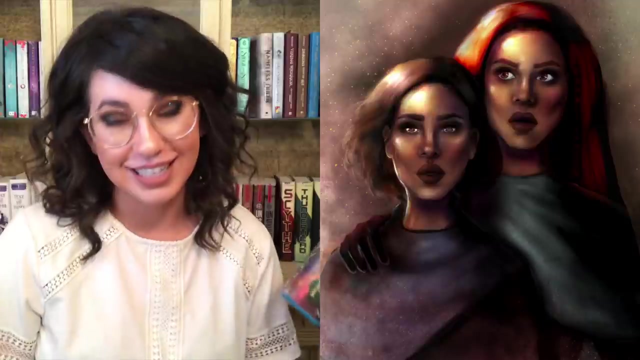 as lesser and often forced into slavery or servitude of some kind, and she wants to join this rebellion that has phoenixes, which is awesome, and she's just one of those sweet, wholesome characters that you're like, yeah, like you can do it. Her sister Val is crazy, She's so. 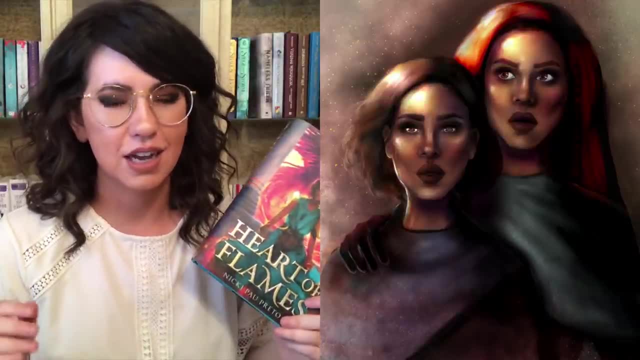 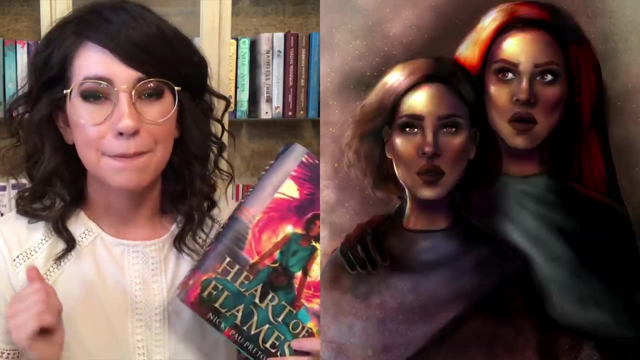 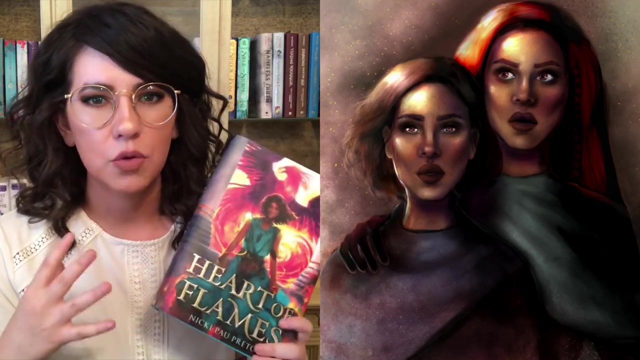 crazy. The things that she does are awful. You see glimpses of that in the first one, but then I think in the second one you really see how crazy she truly is. but because they're sisters and you mostly follow the good one, Veronica, you just always kind of can see the 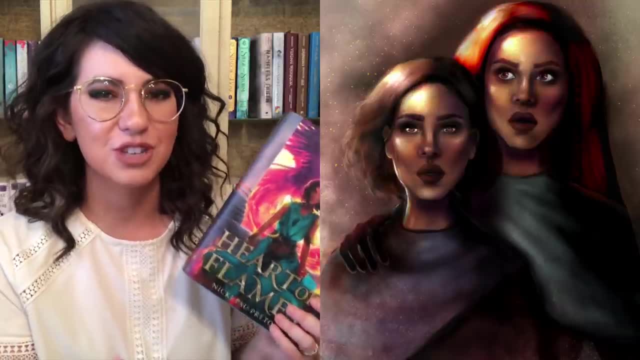 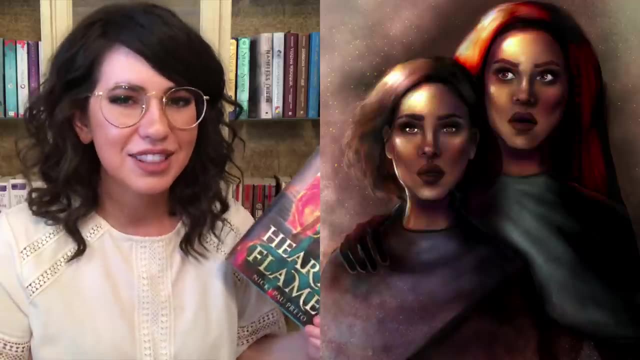 good in Val, but then you know she actually isn't good. You're like: no, she probably should be taken out. you know, Like she, really she, I don't think that she's good for anybody. but then you're like: 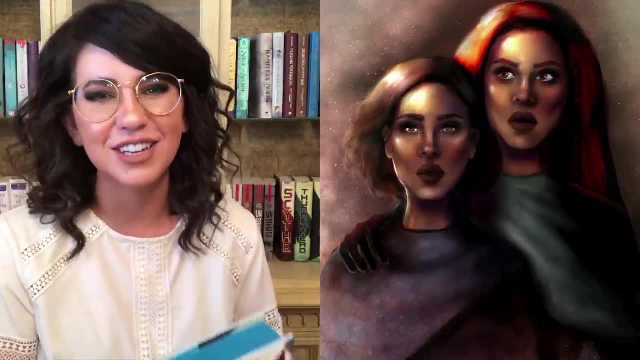 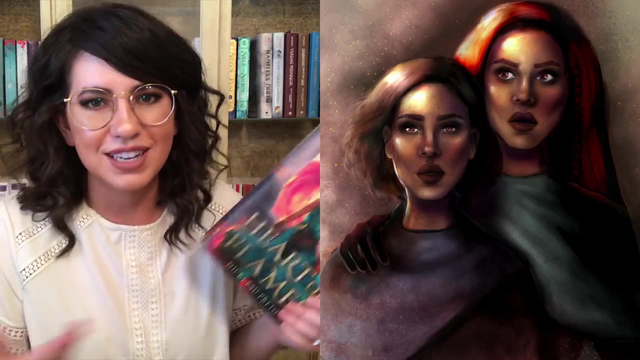 but she's just misunderstood or like she just needs love. you know, Like you try to justify and you definitely see her and I think your feelings toward her are conflicted because you're getting her sister's love for her. I think it's very nicely done And 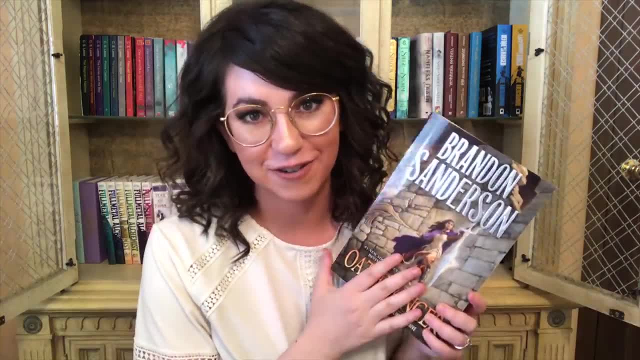 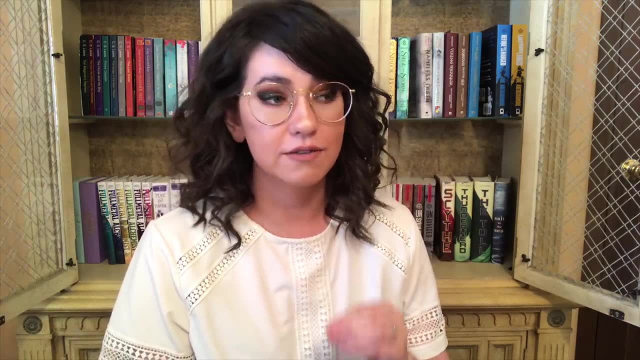 my honorable mention would be Dalinar from the Stormlight Archive by Brandon Sanderson. I absolutely do think a lot of people would consider Dalinar to be one of the main morally gray characters they've come across, but for me there's a specific reason why I don't necessarily agree. 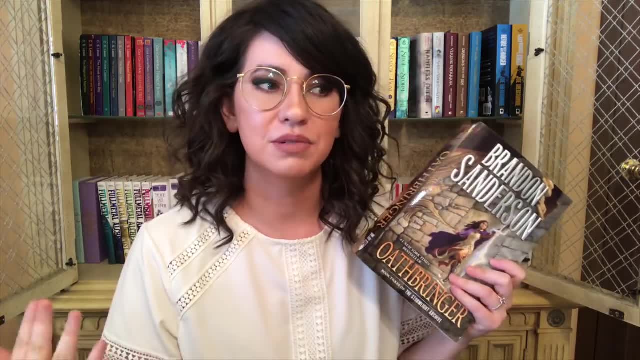 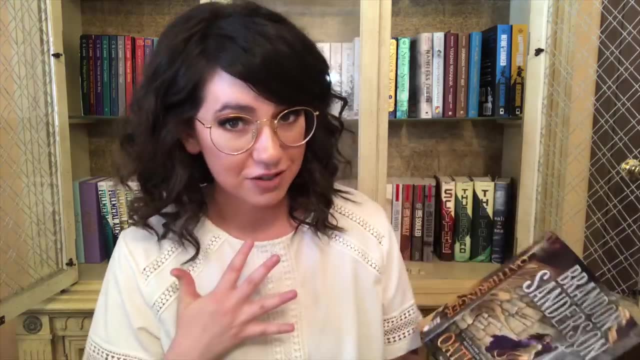 with that, I might actually make an entire dedicated review talking about Dalinar, just him as a character and also the concept of him as a character, and then I might actually make an entire his redemption arc, which I don't really feel like is much of a redemption arc, and I feel like 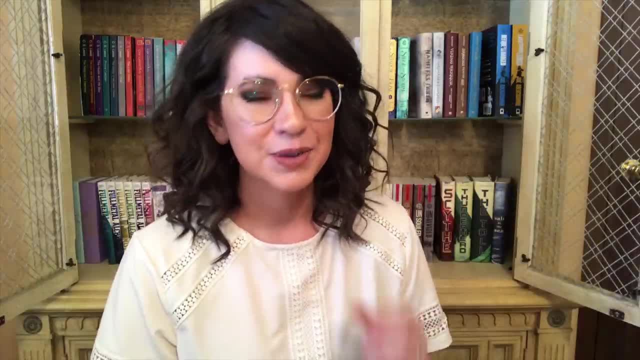 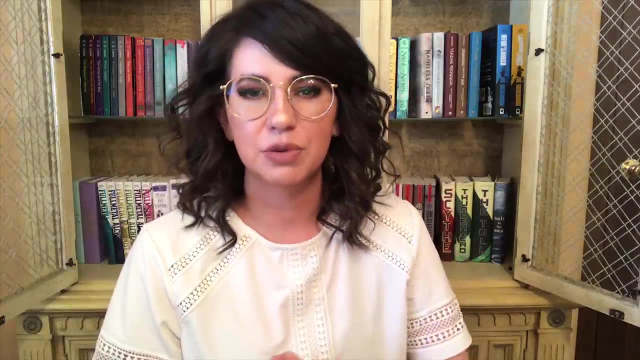 that's kind of controversial if you're a Stormlight Archive fan, but Dalinar is a character that not a spoiler- you know right away from the beginning that he has a reputation as someone known as the Blackthorn, which was this monster on the battlefield during war. And now, when you see him, 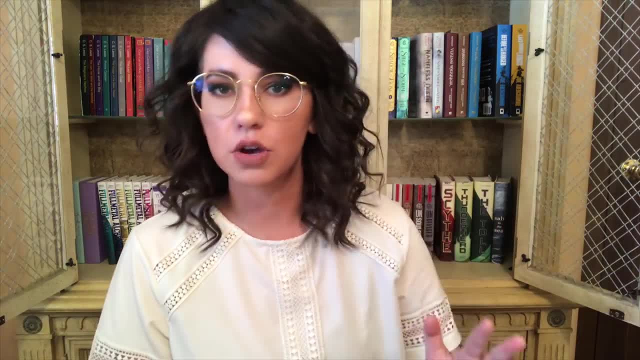 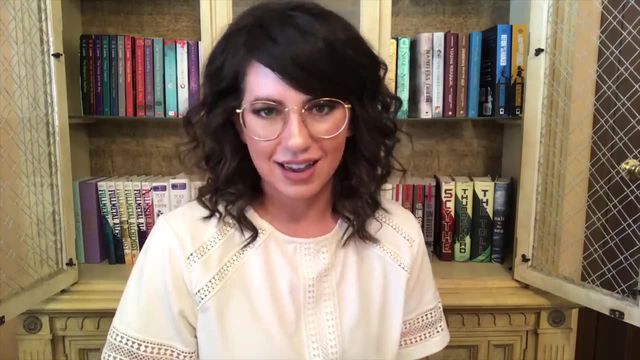 he's all about being honorable and you have to follow the codes and he's all about this honor and everybody's like what happened? This is not how you used to be. What's going on? Where's that monster? We need that guy back And he's like: no, the codes, Be respectful. That's his thing. But he kind of has some memory loss so he's like: I don't really remember what I was like before, And then eventually you find out, And then it's like, oh my gosh, you really. 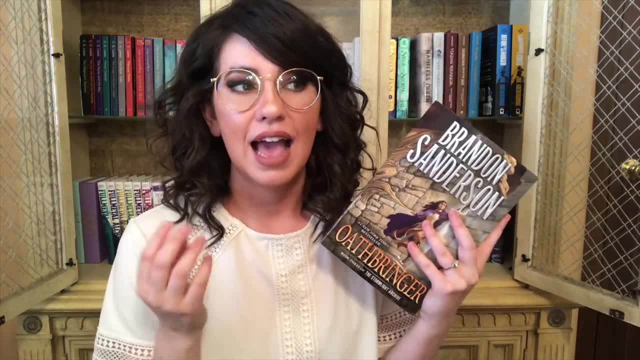 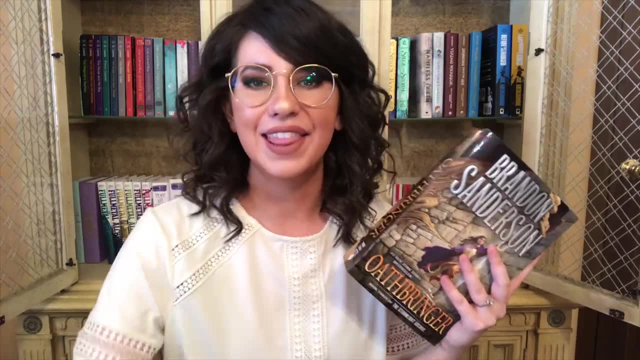 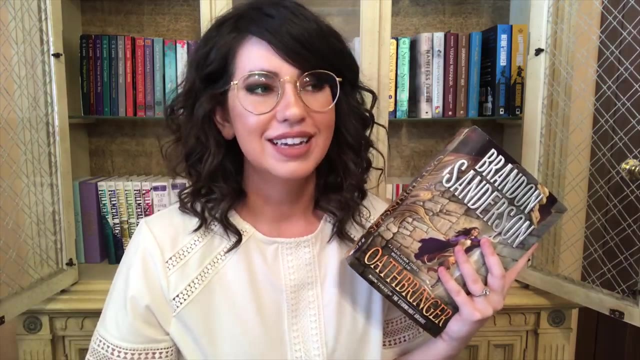 were a monster. As a reader, I think it's really amazing to see him presented to you initially as the person he's become and then see him back how he used to be, Because then you're like: can I root for you? Oh my gosh, you were terrible, And I think it's really cool to see that in. 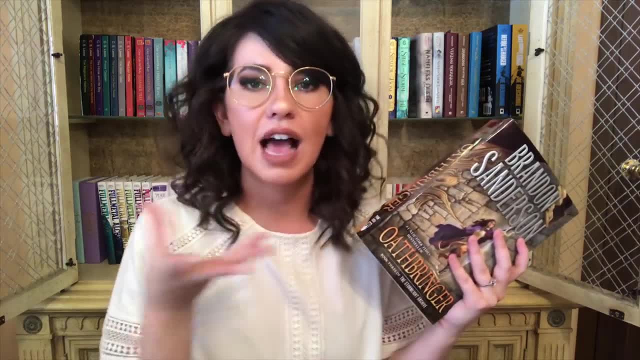 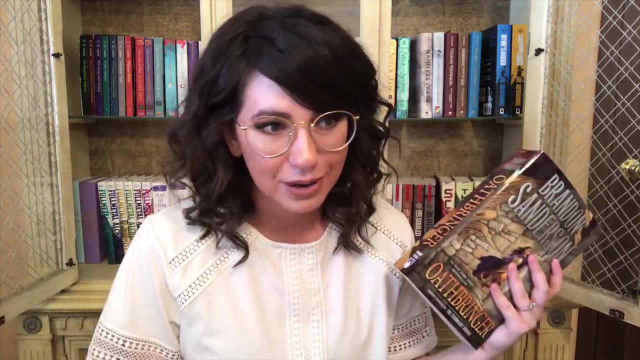 reverse. Usually we see them be terrible and then you find yourself liking them more as the story progresses. Kind of like a Jamie Lannister type character, which the only reason he's not on this list is because I only ever watched the show. I didn't read the books, But I feel like it's the 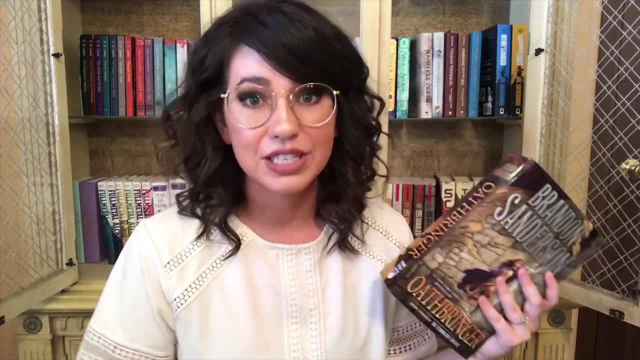 opposite of that. You see him being a character you can root for and being so honorable. and then you see what he did in the past and then, all of a sudden, you're not so sure how you feel about him. It's an honorable mention. 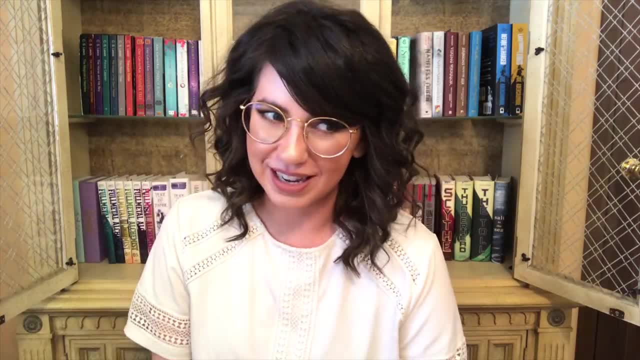 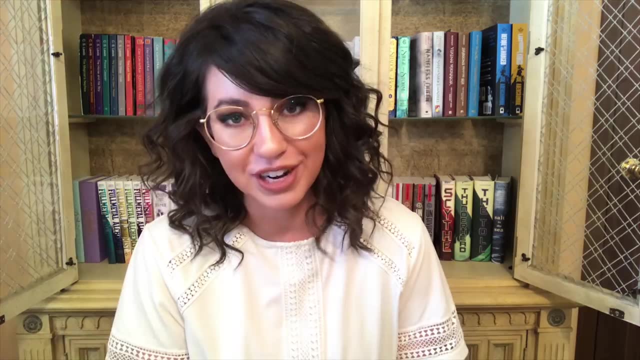 For sort of kind of spoiler reasons, let me know if you want me to do a dedicated video. I kind of want to. That's it for some of my favorite Morley Gray characters. Definitely, let me know who some of your favorite Morley Gray characters are. Are they any of the ones that I mentioned Are there? 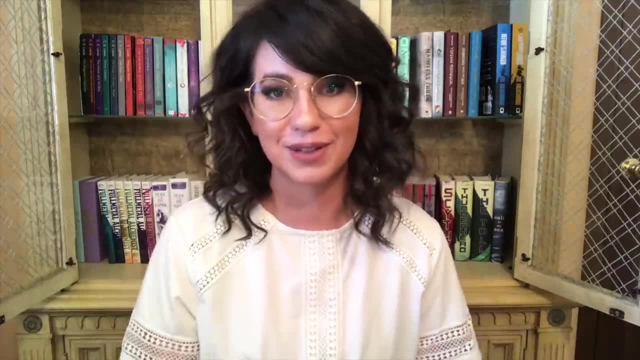 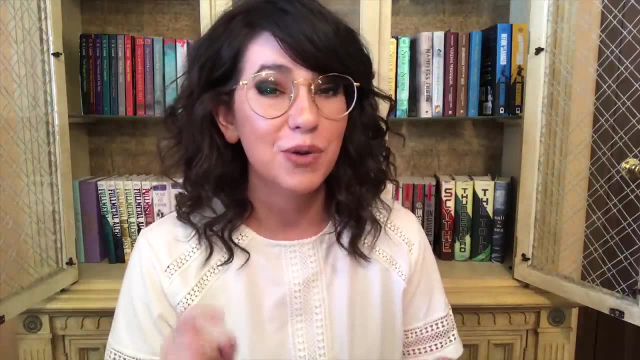 some that are like: how did you leave this one character off? What's wrong with you? I'm excited to see who your favorites are. If there are some that I've never heard of, I'm definitely going to want to know what books they're from. So if you guys don't mind, let me know the book as well as.